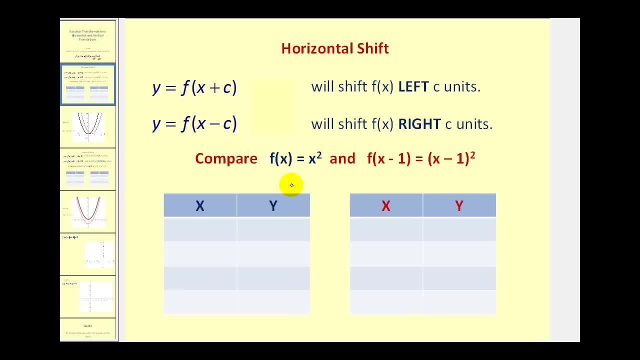 One way to get a feel for this would be to compare a table of values for f of x and f of the quantity x minus one. So let's go ahead and do that, Let's choose. x equals one, two, three, four. So to find y, we just square. 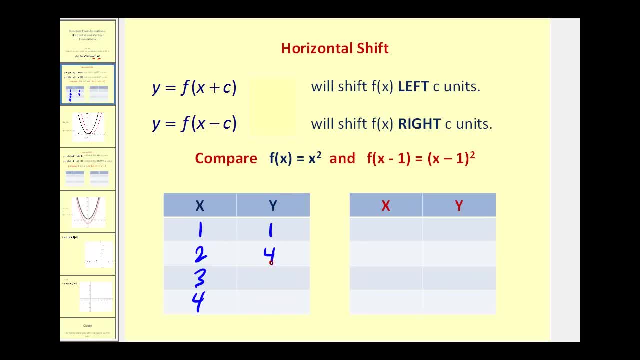 x for f of x. So this would be one squared or one, two squared, which is four, two squared is nine, and four squared is sixteen. Let's use the same x values for f of x minus one. So now we're going to subtract one from the input and then square it. 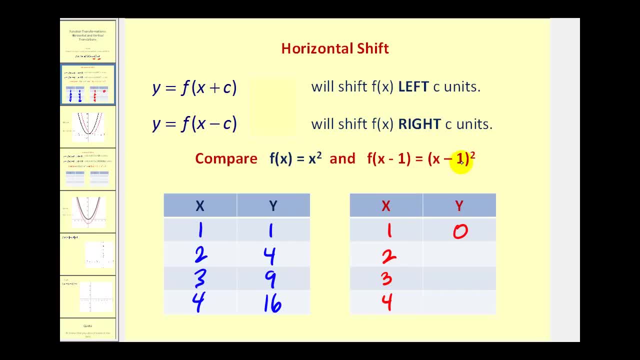 So one minus one squared would be zero. Two minus one squared would be one squared or one. Three minus one squared would be two squared or four. Four minus one squared would be three squared or nine. So if we compare the y values of one, four and nine, 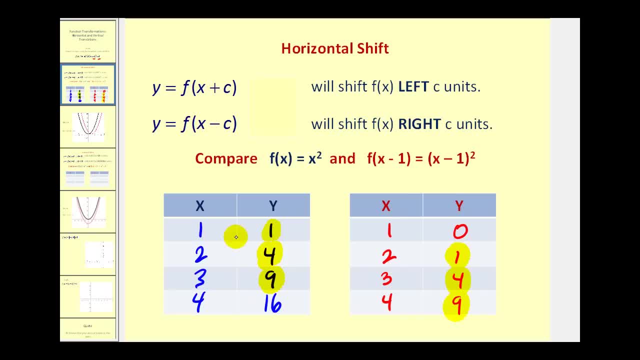 notice that for f of x minus one, we have to increase x by one in order to get the same y value. And when we increase x by one we're shifting the function to the right. So when we subtract a number from x, it moves to the right, And when we add 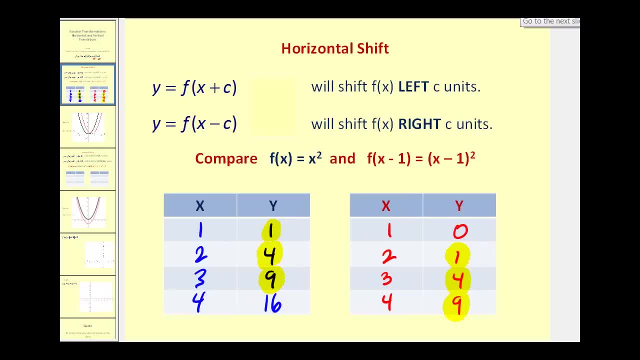 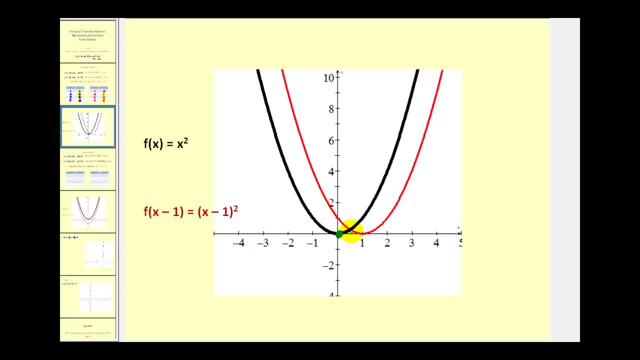 a value to x, it shifts to the left. Here's the graph of these two functions And what you'll notice is, for any corresponding point, let's say the vertex on the original function and the vertex on the shifted function. it's one unit to the right. Pick any point on the original function. 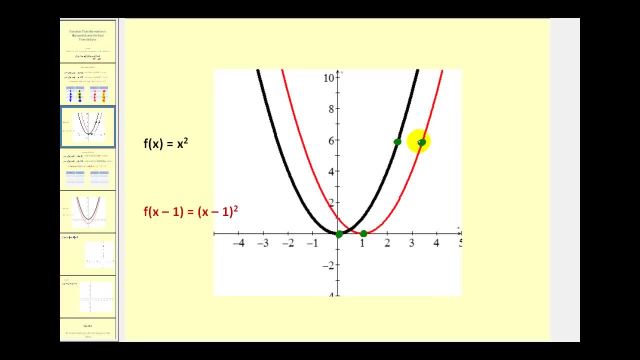 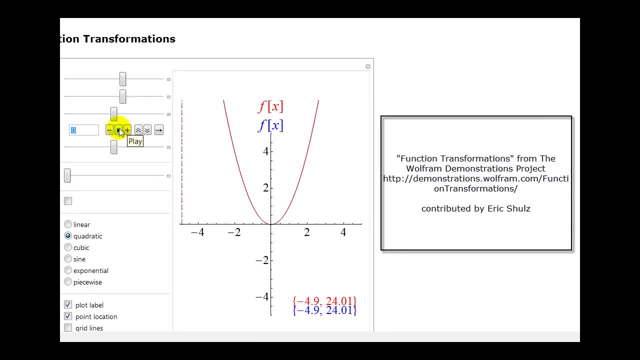 and the translated function will be one unit to the right. Let's look at an animation of this. Here we have an original function in red. As I change the value of c, you'll see the translated function in blue as well as the function notation. 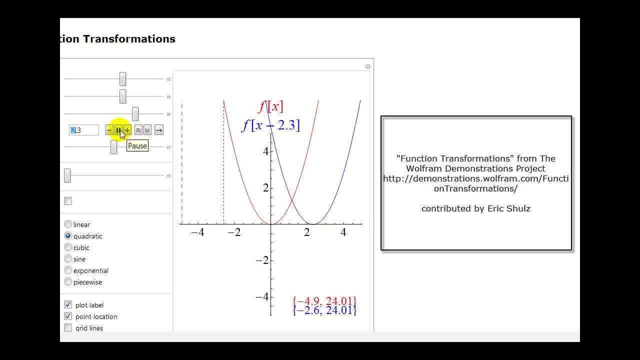 for the translated function. So notice, when it's f of the quantity x minus two point five, the blue function is shifted to the right two point five units. We can also compare corresponding points And what's you'll find is each one in blue is shifted two point five units to the right. 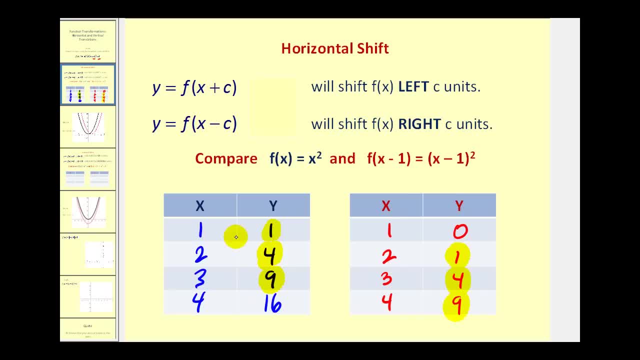 notice that for f of x minus one, we have to increase x by one in order to get the same y value. And when we increase x by one we're shifting the function to the right. So when we subtract a number from x, it moves to the right, And when we add 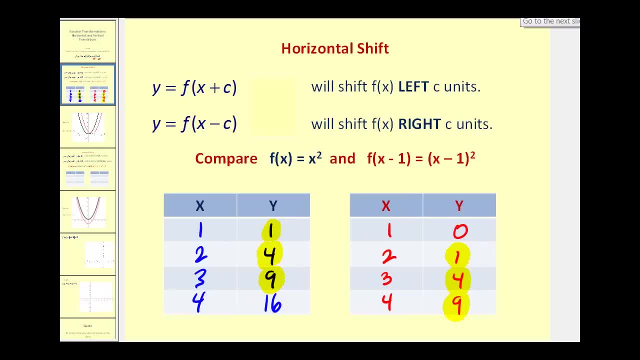 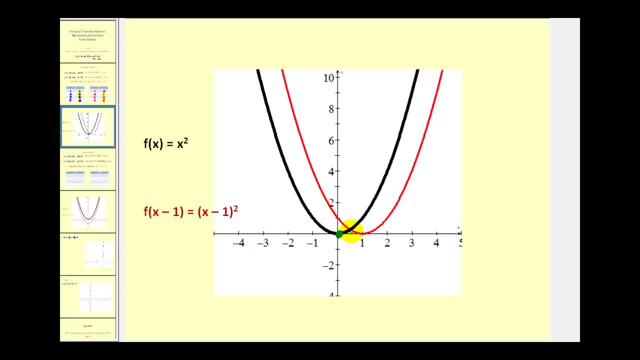 a value to x, it shifts to the left. Here's the graph of these two functions And what you'll notice is, for any corresponding point, let's say the vertex on the original function and the vertex on the shifted function. it's one unit to the right. Pick any point on the original function. 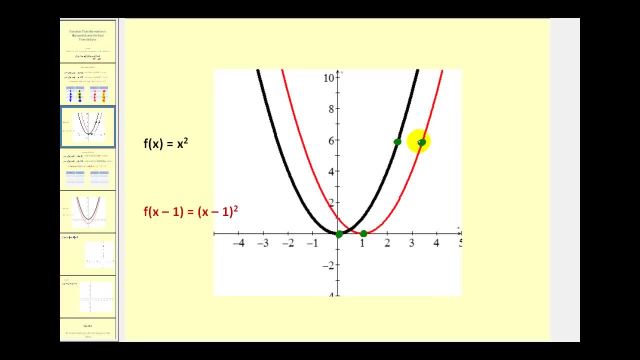 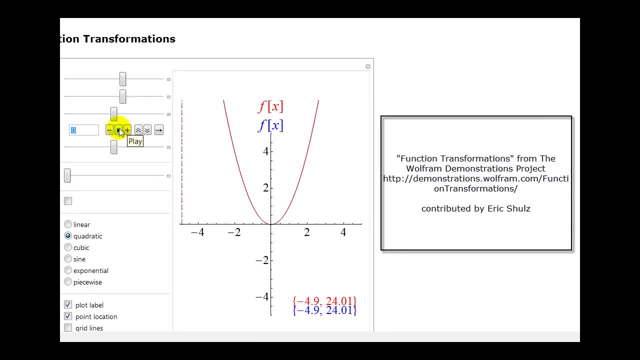 and the translated function will be one unit to the right. Let's look at an animation of this. Here we have an original function in red. As I change the value of c, you'll see the translated function in blue as well as the function notation. 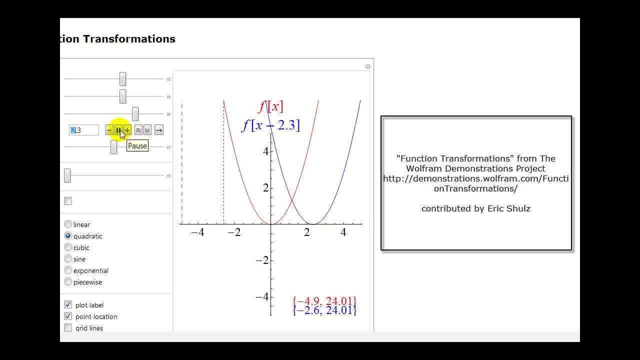 for the translated function. So notice, when it's f of the quantity x minus two point five, the blue function is shifted to the right two point five units. We can also compare corresponding points And what's you'll find is each one in blue is shifted two point five units to the right. 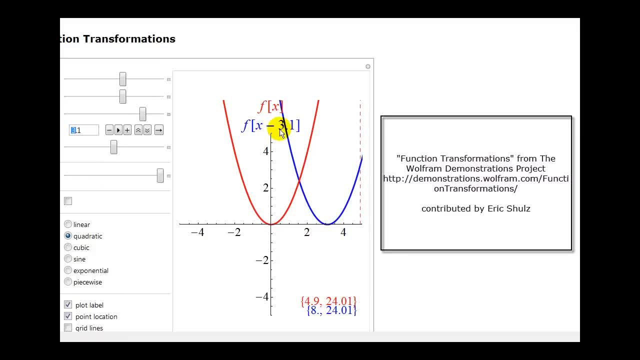 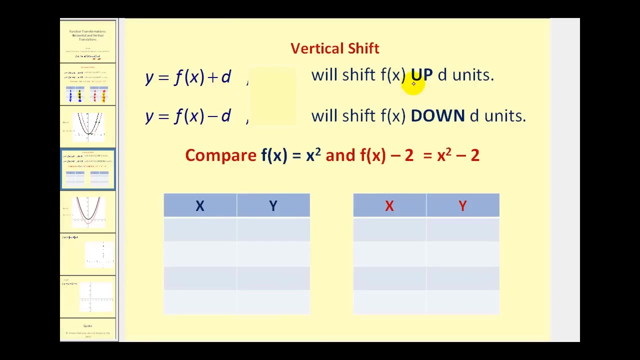 Let's go and see what happens when we change this to x plus a constant. You can see when we have f of x plus one, the translated function is shifted to the left. now Let's go and talk about a vertical shift. now y equals f of x plus d will shift f of x. 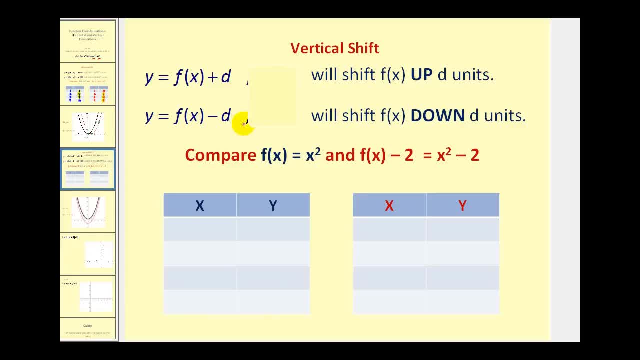 up d units And y equals f of x minus d will shift f of x down d units And this translation probably seems more logical. Remember: f of x is equal to y, So if we add d units to y, the function will shift up. 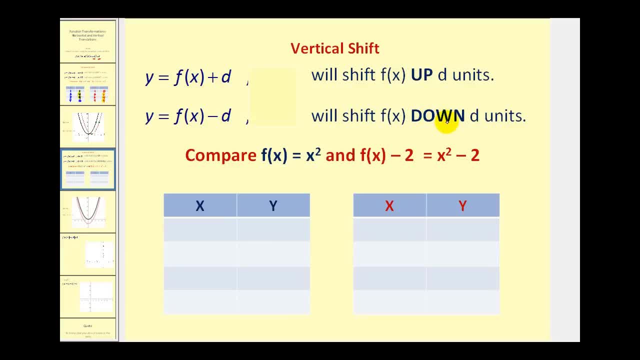 And if we subtract d units from y, the function would shift down. Let's go ahead and do another comparison using f of x and f of x minus two. So again, for f of x, we'll just square the input. So we'll have one, four, nine, sixteen. 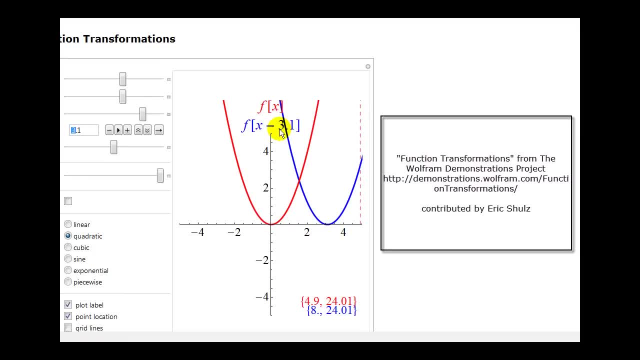 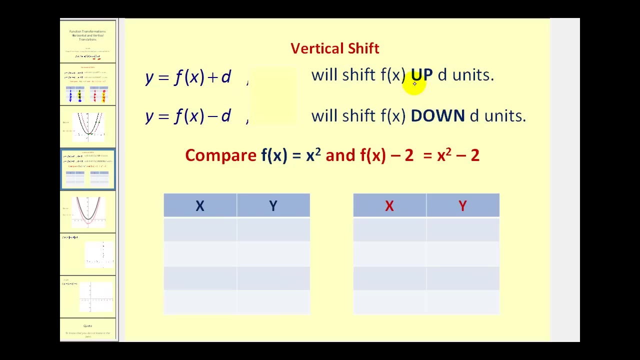 Let's go and see what happens when we change this to x plus a constant. You can see when we have f of x plus one, the translated function is shifted to the left. now Let's go and talk about a vertical shift. now y equals f of x plus d will shift f of x. 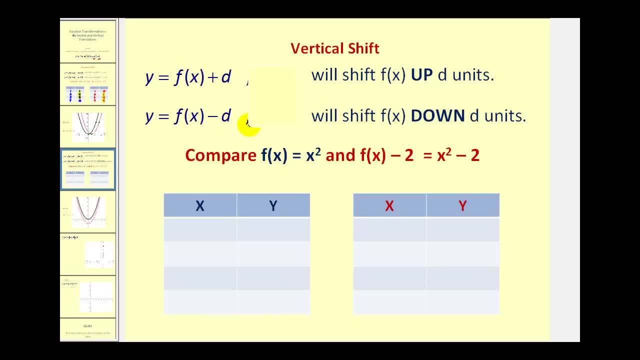 up d units And y equals f of x minus d will shift f of x down d units And this translation probably seems more logical. Remember: f of x is equal to y. So if we add d units to y, the function will shift. 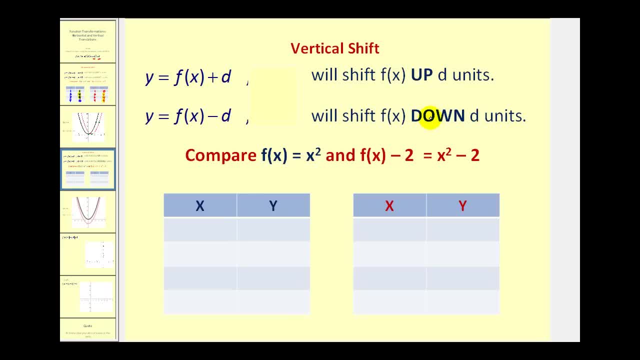 up, And if we subtract d units from y, the function would shift down. Let's go ahead and do another comparison using f of x and f of x minus two. So again for f of x, we'll just square the input. So we'll have one, four, nine, sixteen. 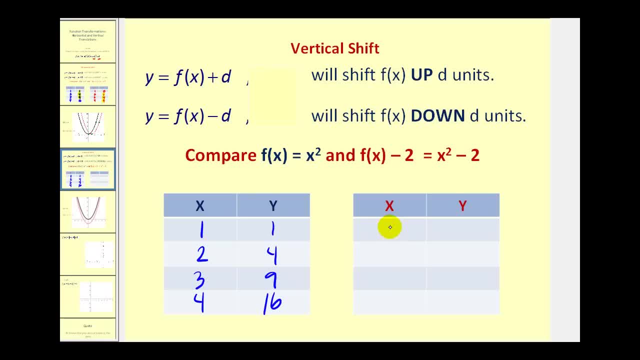 For f of x minus two, we'll use the same inputs, But now we'll square the input and then subtract two. One squared minus two would be negative one. Two squared minus two, that would be four minus two or two. Three squared minus two, that would be nine minus two or seven. 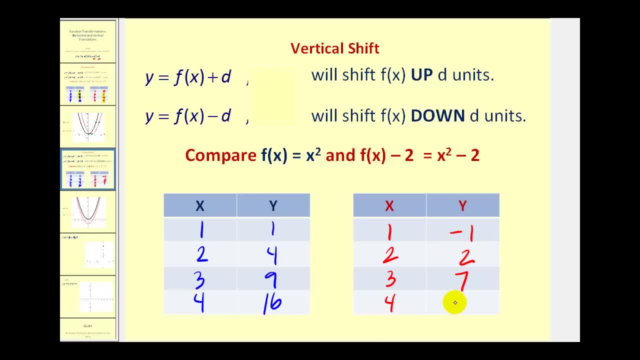 And four squared minus two would be sixteen minus two or fourteen. So if we do another comparison of the y values of the function, notice that all of the y values in red are two less than the y values in blue. Therefore this function would be two units lower. 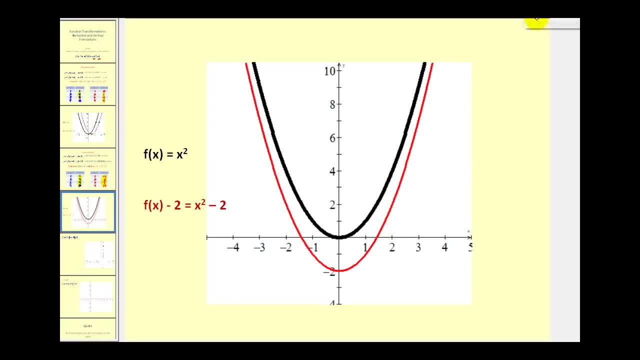 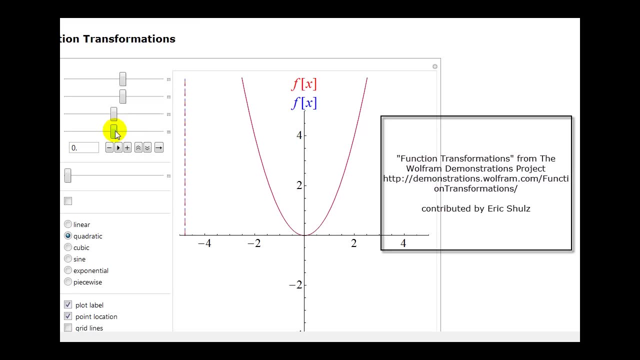 than the original. Here's the graph of those two functions, And so we can pick any point on the original black function and to find the corresponding point on the translated function, we would just move this point down two units. Let's go and take a look at an animation of this as well. So as we change the value of 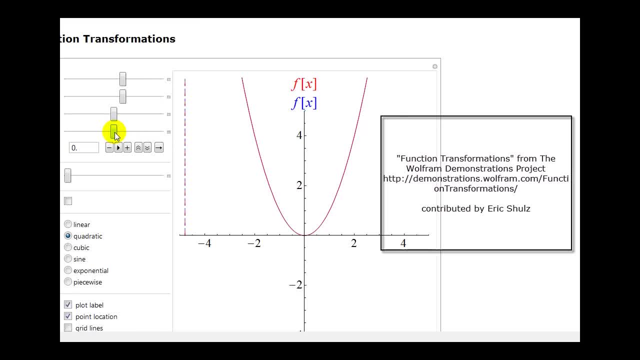 d, we'll see how it affects the graph. The translated graph will be in blue. As we increase d, the function is shifted upward, And if we have f of x minus d, the function is shifted down from the original. Let's go and take a look at some examples. 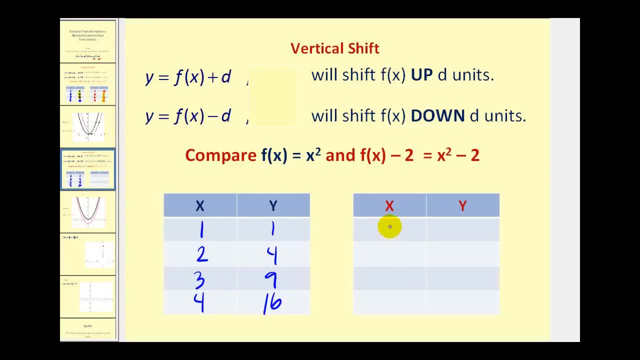 For f of x minus two, we'll use the same inputs, But now we'll square the input and then subtract two. One squared minus two would be negative one. Two squared minus two, that would be four minus two or two. Three squared minus two, that would be nine minus two or seven. 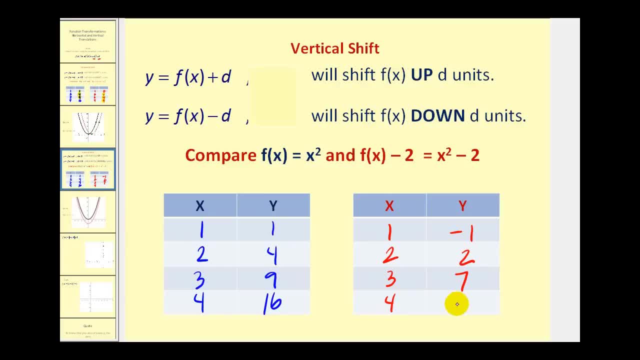 And four squared minus two would be sixteen minus two or fourteen. So if we do another comparison of the y values of the function, notice that all of the y values in red are two less than the y values in blue. Therefore this function would be two units lower than the original. 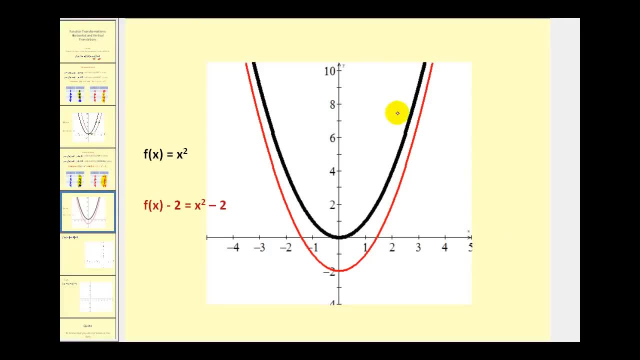 Here's the graph of those two functions, And so we can pick any point on the original black function And to find the corresponding point on the translated function, we would just move this point down two units. Let's go and take a look at an animation of this as well. So as we change the value of d, 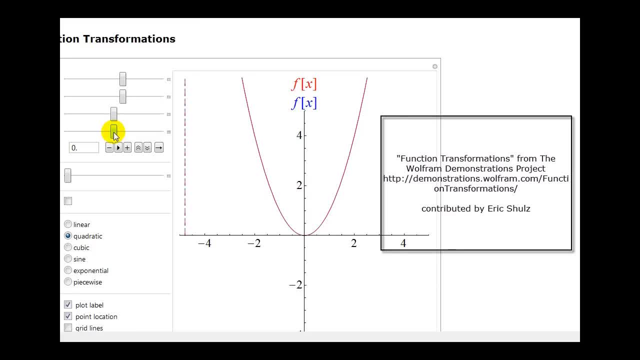 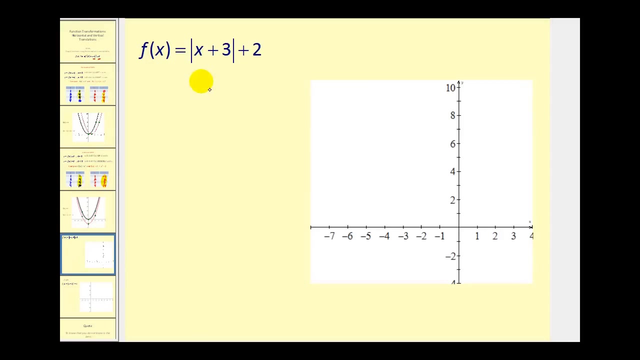 we'll see how it affects the graph. The translated graph will be in blue. As we increase d, the function is shifted upward, And if we have f of x minus d, the function is shifted down from the original. Let's go and take a look at some examples. We want to be able to use what we just learned. 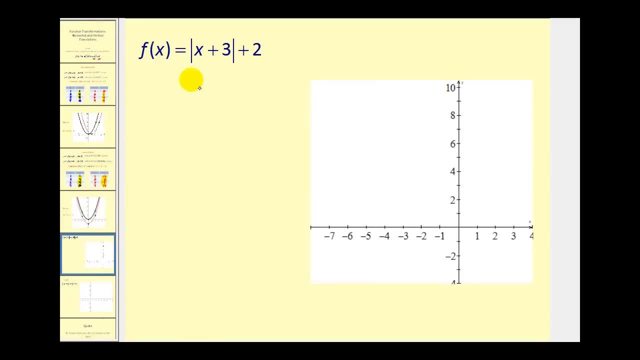 in order to accurately and quickly graph f of x equals the opposite value of the quantity x plus three plus two. So the first thing we need to do is recognize what the parent function is, And in this case it would be the absolute value of x. 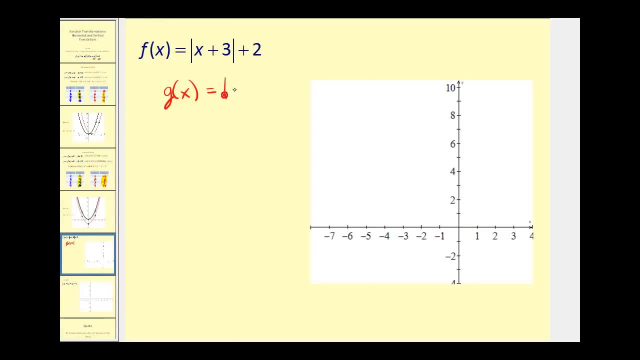 So let's go ahead and call g of x equals the absolute value of x. Let's go ahead and graph this for reference. Remember, the absolute value function forms of v looks something like this: Let's go ahead and identify a few of these points. 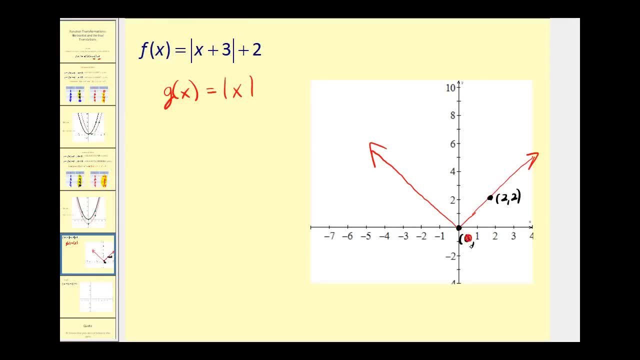 This would be two two. This would be zero, zero, And this would be negative two two. The next thing we need to be able to do is recognize how taking the absolute value of x plus three and then adding two would translate the parent function. So what we could do is say that f of x. 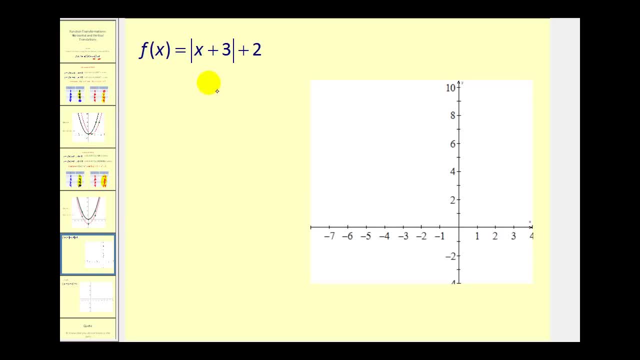 We want to be able to use what we just learned in order to accurately and quickly graph. f of x equals the absolute value of the quantity x plus three plus two. So the first thing we need to do is recognize what the parent function is, And in this case it would be the absolute value of x. So let's go ahead and call g of x. 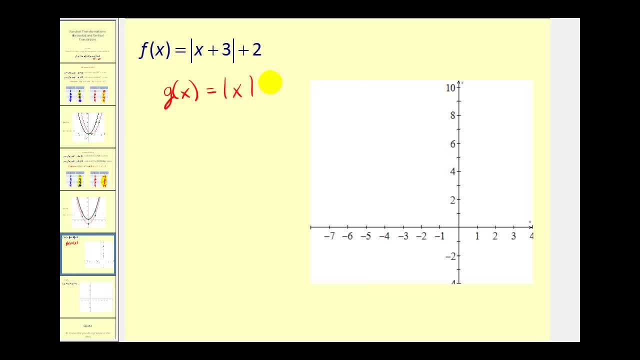 equals the absolute value of x. Let's go ahead and graph this for reference. Remember, the absolute value function forms a, v. It looks something like this: Let's go ahead and identify a few of these points. This would be two, two. This would be zero, zero. 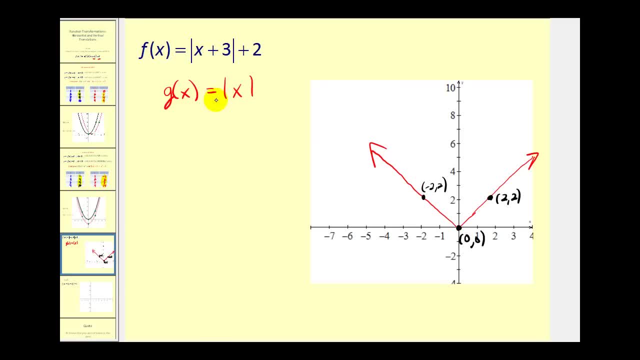 And this would be negative two, two. The next thing we need to be able to do is recognize how taking the absolute value of x plus three and then adding two would translate the parent function. So what we could do is say that f of x is equal to g of 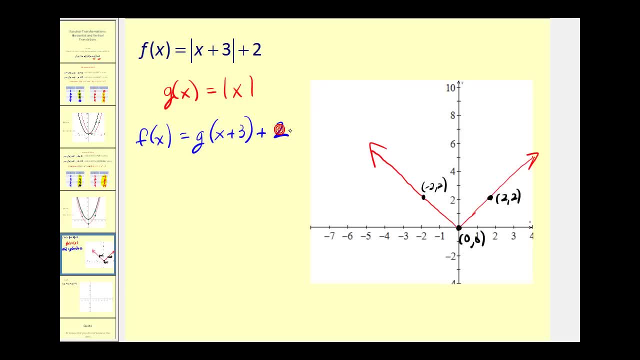 x plus three plus two, if that's helpful. Notice: if g is just the absolute value of x, g of x plus three would be this part of the function And then the plus two would be the constant on the end, So increasing x by three here. 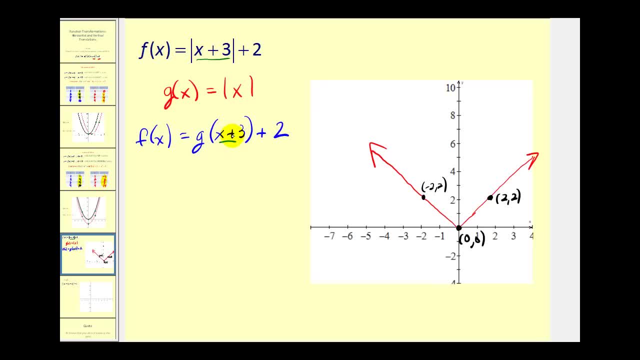 which would be the same as the x plus three here would shift the graph left three units. Then, adding two to the absolute value function here or here would shift the function up two units. So now what we can do is take these three key points and shift them. 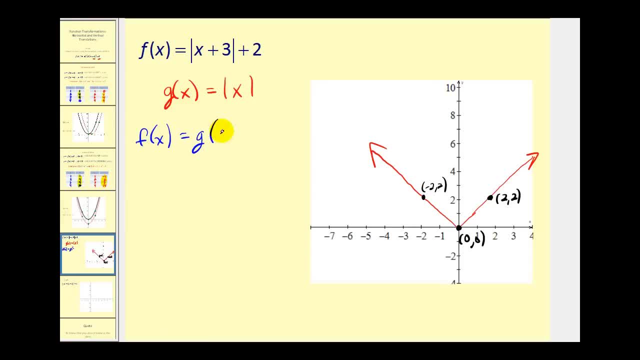 is equal to g of x plus three plus two, if that's helpful. Notice: if g is just the absolute value of x, g of x plus three would be this part of the function And then the plus two would be the constant on the end. 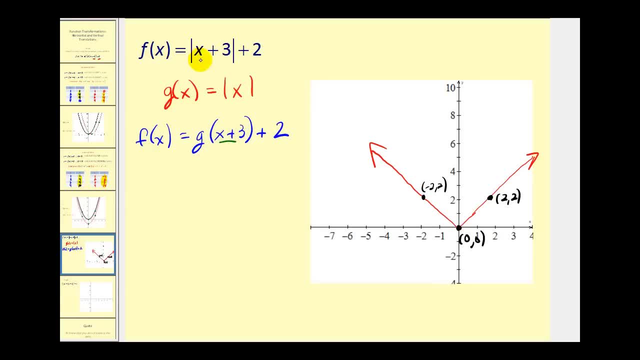 So increasing x by three here, which would be the same as this x plus three here, would shift the graph left three units. Then adding two to the absolute value function here or here would shift the function up two units. So now what we can do is take these three key points. 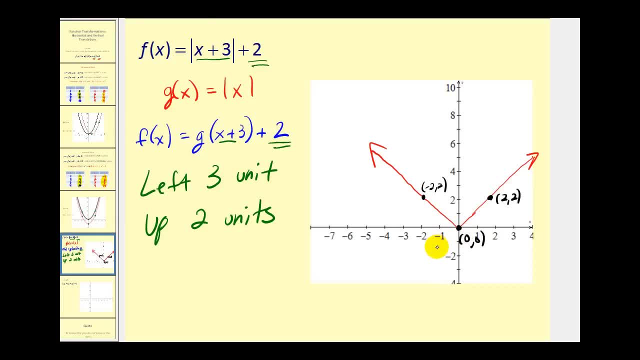 and shift them- left three units and up two- to graph the given function. So let's do that. Let's start with the leftmost point. We're going to go left three points, Left three units and then up two, So we'd be over to negative five. 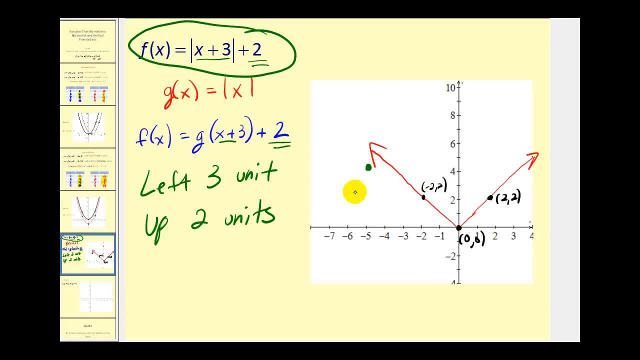 and then up to four. Next, we take this point zero, zero and shift it left three units and up two. We'd be here at negative three, two. And lastly, we'll take this rightmost point: shift it left three units and up two. 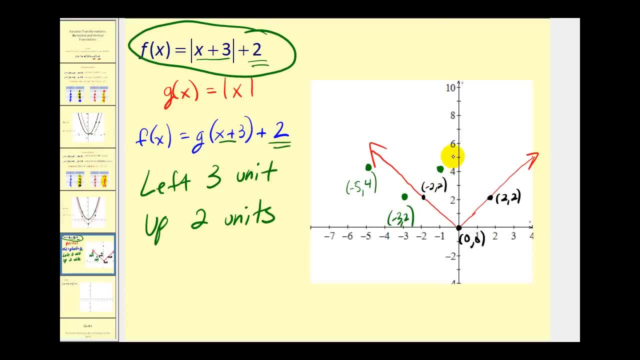 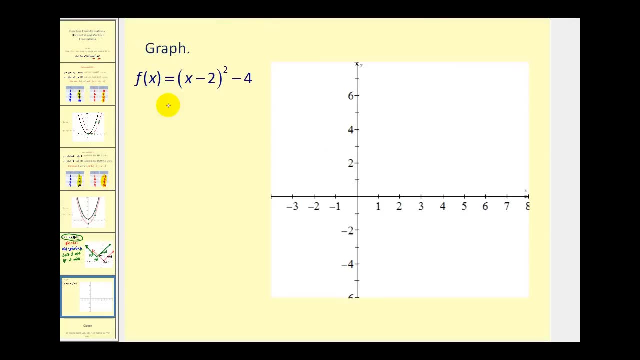 And we'd be right here at negative one. four: Now that we know that the absolute value function is a v-shape, we can form the new function here in green using translations, And it looks something like that: Let's go ahead and try another one. 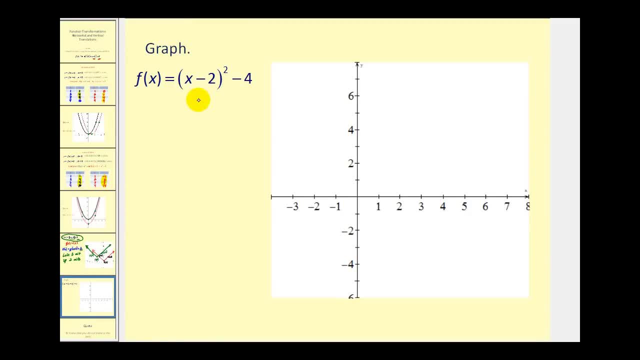 Again, the first step is going to be to recognize what the parent function would be. If f of x equals the quantity x minus two squared minus four, we should recognize the parent function as let's call it: g of x equals x squared. So if we want to create f of x, 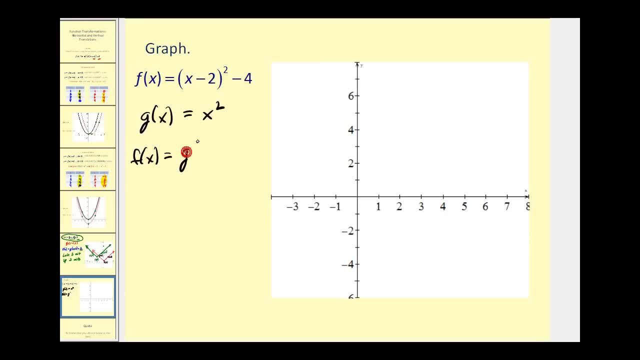 using g of x, f of x is going to equal g of well, x minus two is being squared, so we'd have g of x minus two, and then we're subtracting four. Now, after a while you may not have to write it like this, but it may help at the beginning to recognize. 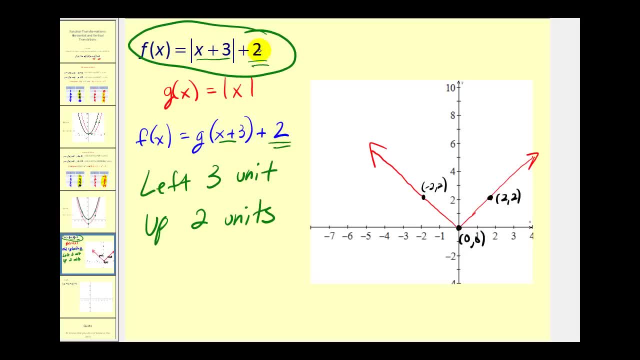 left three units and up two to graph the given function. so let's do that. Let's start with the left two, leftmost point. we're going to go left three units and then up two, so we'd be over to negative five. 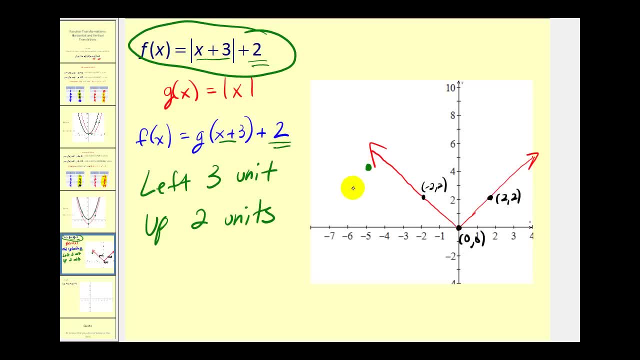 and then up to four. Next, we take this point zero, zero and shift it left three units and up two. We'd be here at negative three, two. And lastly, we'll take this rightmost point: shift it left three units and up two. 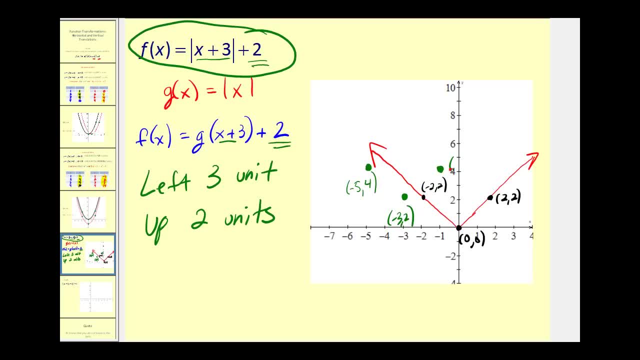 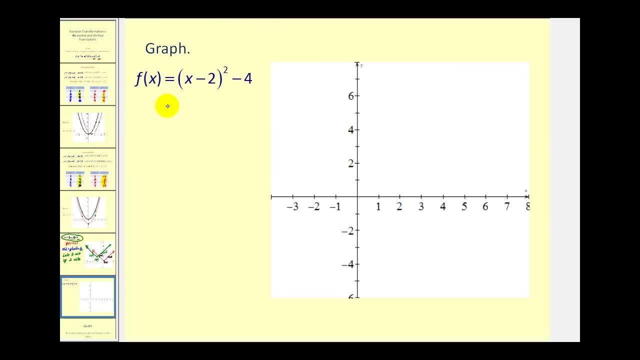 so we'd be right here at negative one. four: Now that we know that the absolute value function is a v-shape, we can form the new function here in green using translations, And it looks something like that: Let's go ahead and try another one. 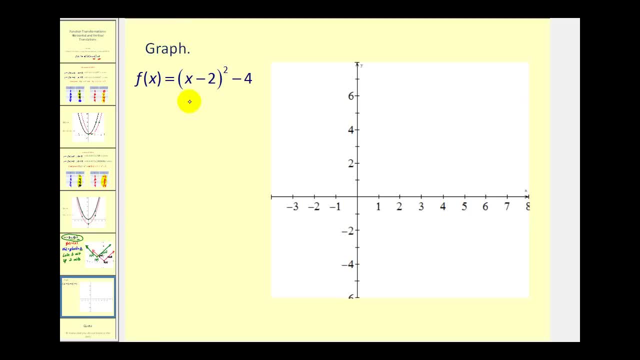 Again, the first step is going to be to recognize what the parent function would be. If f of x equals the quantity x minus two squared minus four, we should recognize the parent function as let's call it: g of x equals x squared. 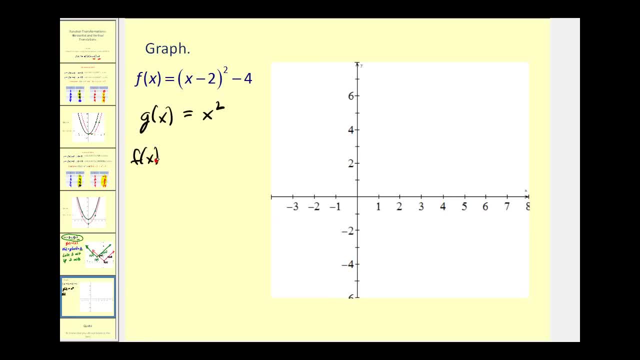 So if we want to create f of x using g of x, f of x is going to equal g of well, x minus two is being squared, so we'd have g of x minus two, and then we're subtracting four. 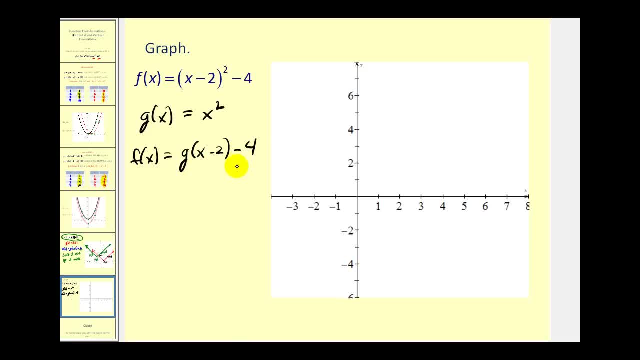 Now, after a while, you may not have to write it like this, but it may help at the beginning to recognize that here we're decreasing the input of x by two, which means it will shift it right: two units, Recognizing this x minus two here. 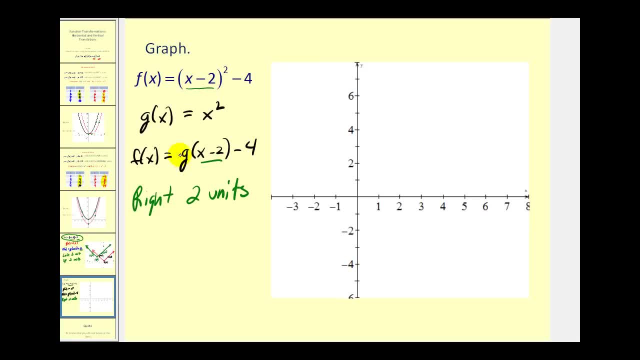 is the same as the x minus two here, And then subtracting four from this function value would shift it down four units. So this minus four is the same as this minus four here in the given function. So to graph this given function we should first sketch the graph of the parent function. 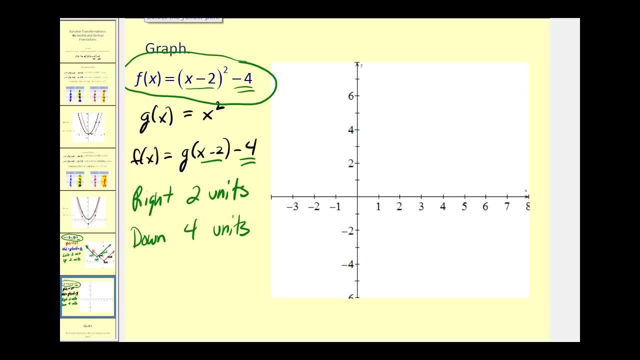 g of x equals x squared. Let's go ahead and do that. Remember that's a parabola with its vertex at the origin. This would be the vertex: One squared would be one, two squared would be four. One squared would be one, two squared would be four. 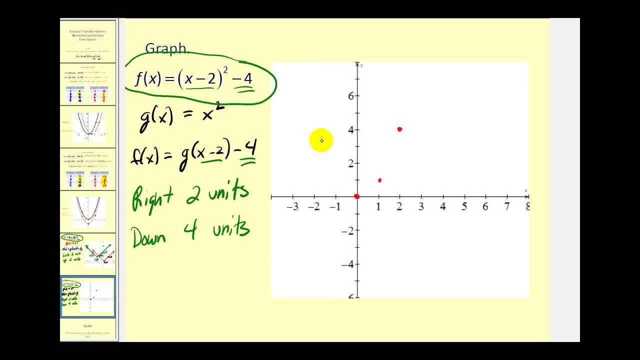 One squared would be one, two squared would be four, And then we have a mirror image on the other side of the y-axis. So we have a point here and a point here. So this is the parent function, And what we're going to do now is pick some key points here. 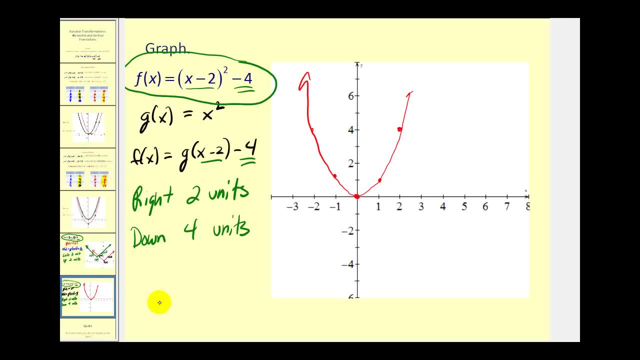 and then shift each of them right two units and down four units. So let's start with the vertex. We'll shift it right two units and down four units to here. Next, we'll take this point here and shift it right two units. 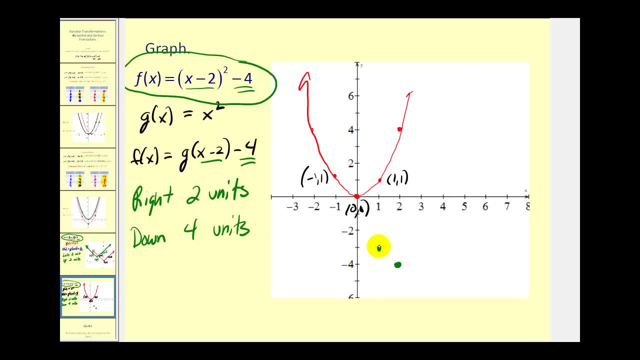 And down four units. that would be here at one negative three. Then we'll take the point one one, shift it right two and down four. here Might as well go ahead and do these last two points. Let's take this one and shift it to the right two. 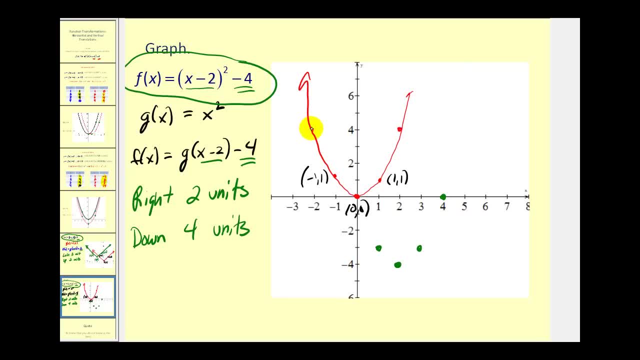 Down four would be here on the x-axis And the same here. shift it right two and down four. We'd be at the origin now. So the translated function would be this green parabola as we see here. All right,